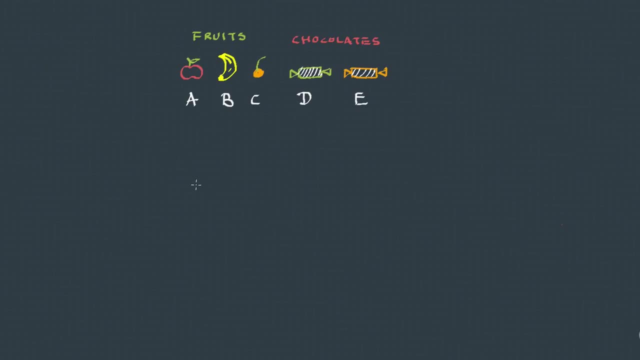 Here we have three fruits: apple, banana and cherry- and two chocolates: dairy milk and eclairs. If I am asked to choose a fruit or a chocolate, I would do it in this way. So the set with my choice of selection will be either apple or banana, or cherry or dairy. 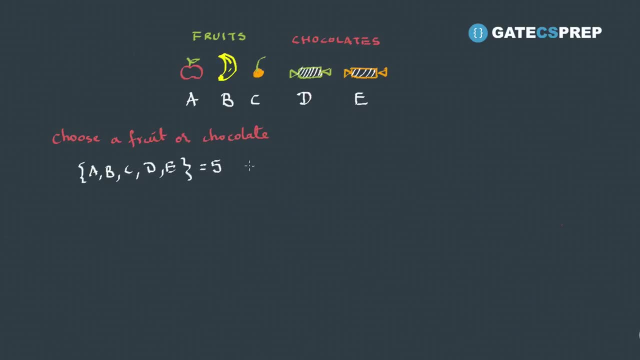 milk or eclairs, So I can select in five different ways. Now what if I am asked to select a fruit and one chocolate? Then, since it is a fruit and a chocolate, I would do it this way: Maybe I pick up an apple, then a dairy milk or apple with eclairs, Otherwise banana and dairy. 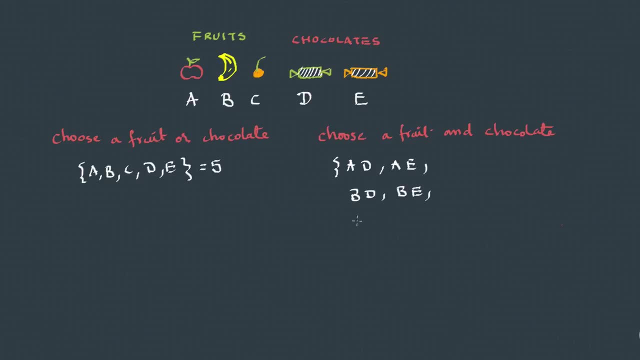 milk or banana and eclairs and the other two Cherry and dairy milk and cherry and eclairs. So how many different selections are possible? I have one, two, three, four, five and six, If I think, selecting the fruits as event one and selecting the chocolates as event two, and if these two 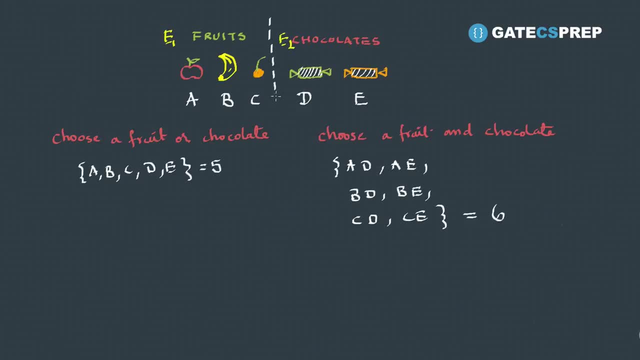 are separate, that is, if there are no common terms and let's assume that this can be done in some m ways and this could be done in some n ways, and if I have to do event one or event two together, we will be using the sum rule, which says that event one or event two. So 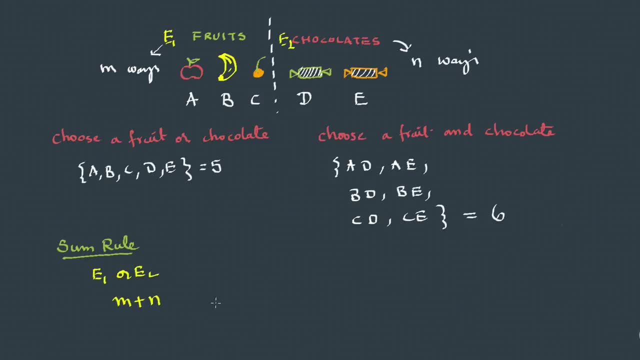 if I have to do event one or event two together can be done in m plus n ways, And if I have to perform event one and event two together, we will be using the product rule, which says that event one and event two together can be done in m into n ways. The sum rule stresses: 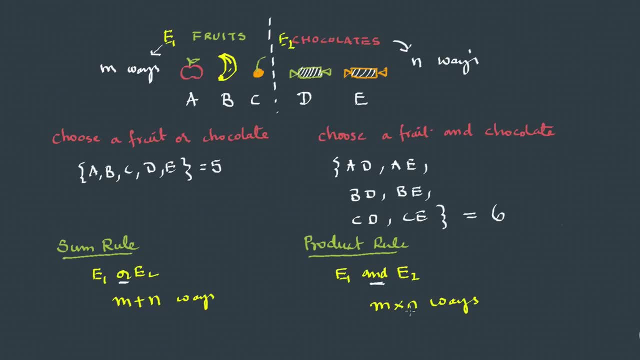 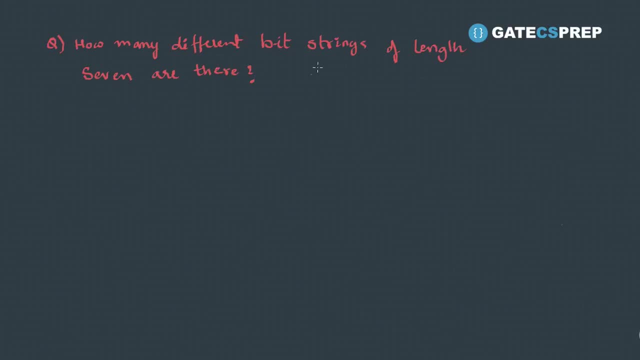 on or, and the product rule stresses on, and Here we have a question: How many different bit strings of length seven are there? So they are saying a string with seven, So let me take this as seven positions. Now the string is a bit string, So it has two possible options.